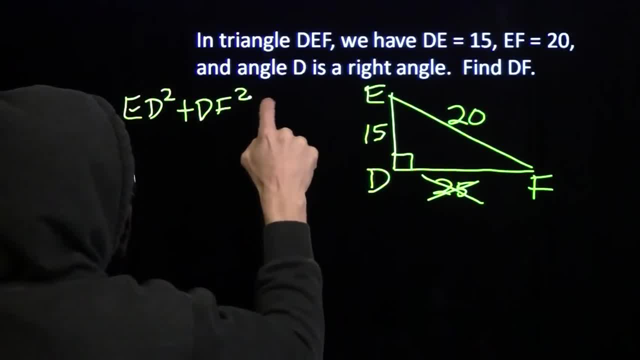 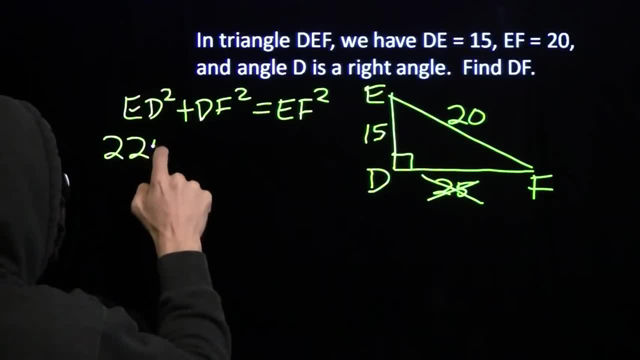 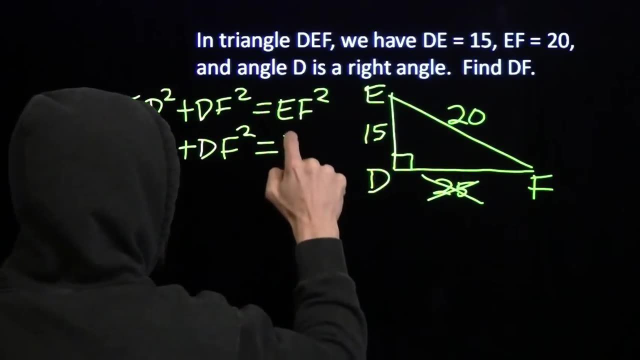 E D squared plus 25 squared Plus D F squared equals E F squared E D is 15, so E D squared is 225 plus D F squared E F is 20.. We square that. we. 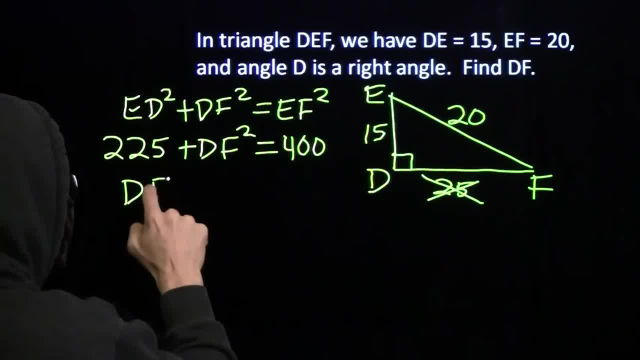 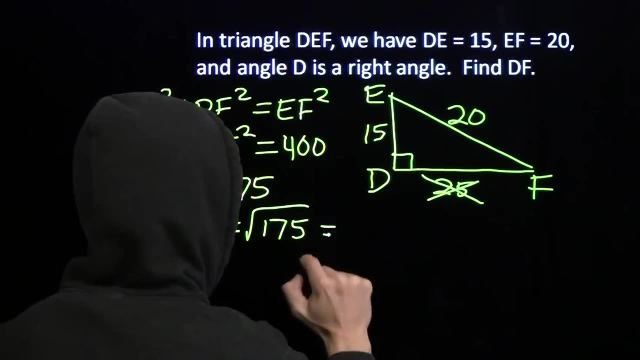 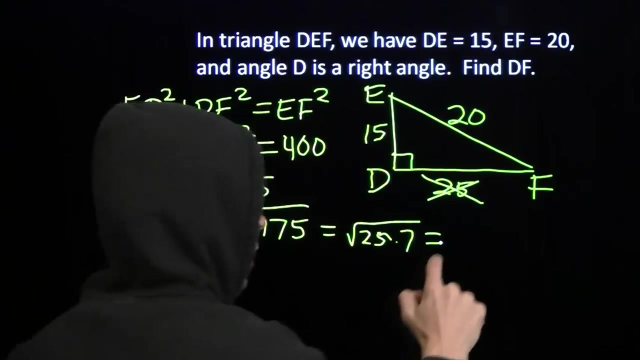 get 400.. So we've got D F squared. Subtract the 225 is 175.. And then we take the square root. We can pull out a factor of 25 from there. Nice, perfect square factor. We have square root of 25 times 7.. Pull out the 5, you have 5 root 7.. 5 root 7 is our answer for D F. 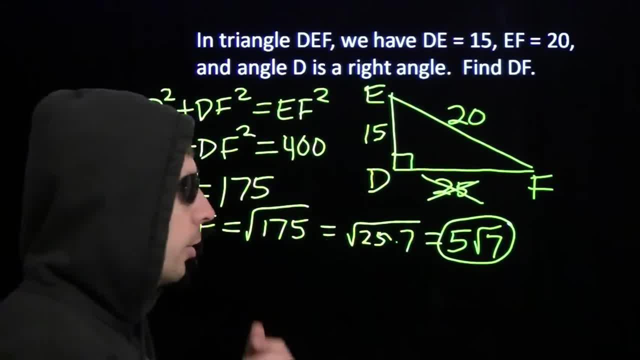 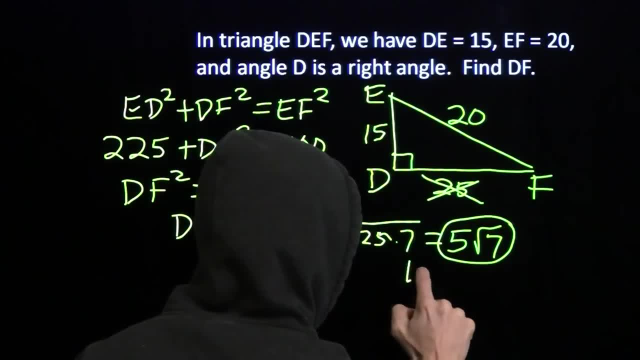 It's not a 3,, 4, 5 triangle. What went wrong here? If we look at our diagram, we can see what we're given So we can move into the right triangle. We can see what's the right triangle We're going. 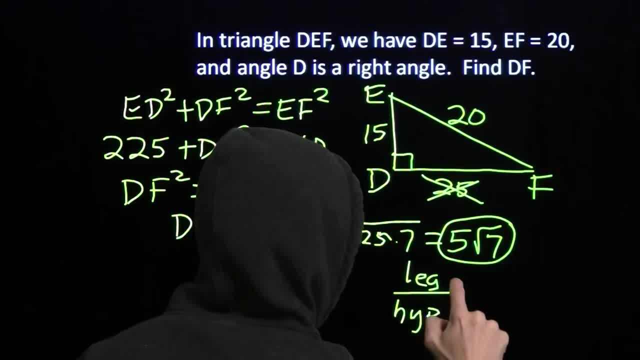 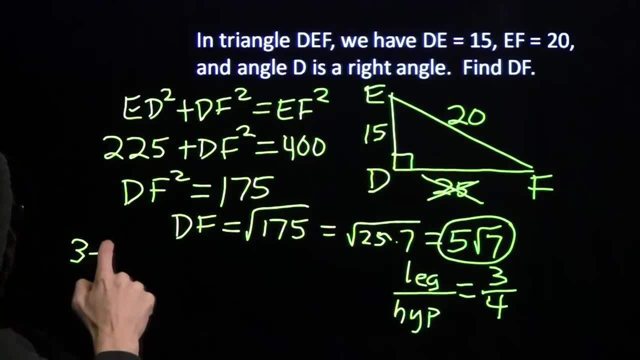 to make a triangle. Now, we're gonna make our triangle. We're gonna make our triangle. What's leg to hypotenuse is 3 to 4.. But in a 3-4-5 triangle, what we're given is leg to leg is 3 to 4.. 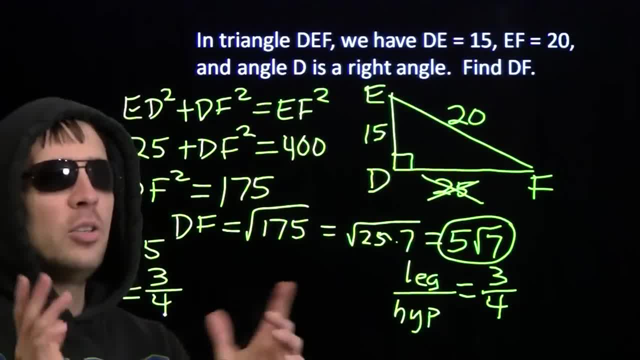 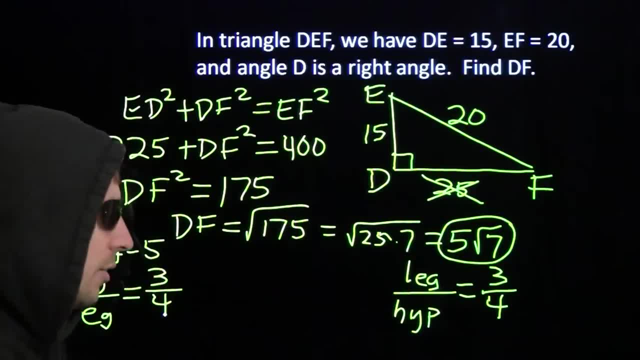 So you have to pay attention. when you've got two sides in the right triangle and you're going to try to use that clever ratio scaling strategy we talked about in the last video, You have to pay attention to which sides you're given Leg to. the hypotenuse is 3 to 4.. 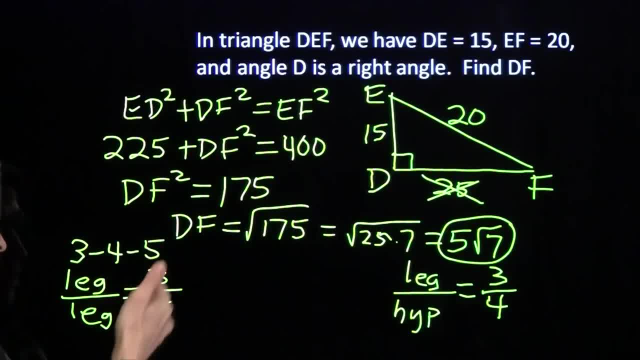 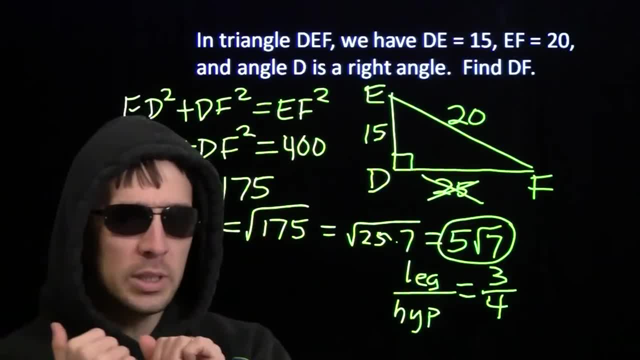 You don't have a 3-4-5 triangle, because in a 3-4-5 triangle it's leg to leg, that's 3 to 4.. So when you're using the Pythagorean triples, solving problems in clever ways like we did, 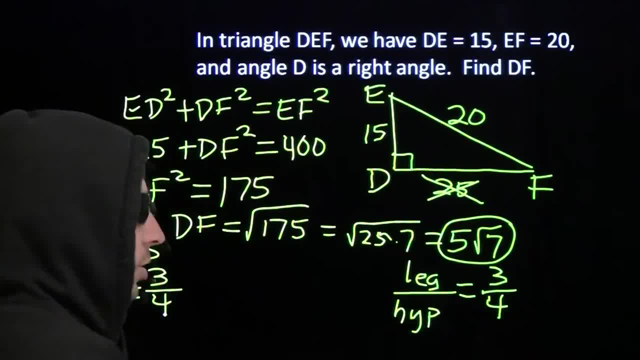 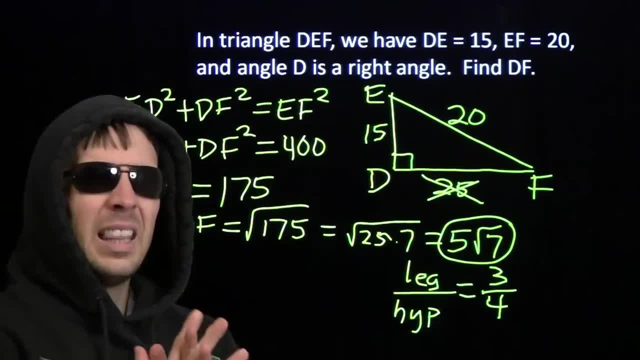 in the last video. you've got to pay very close attention to which sides you're given, And once you've got that down, I want you to think about this problem again, Think about what we have here And think about how you might still 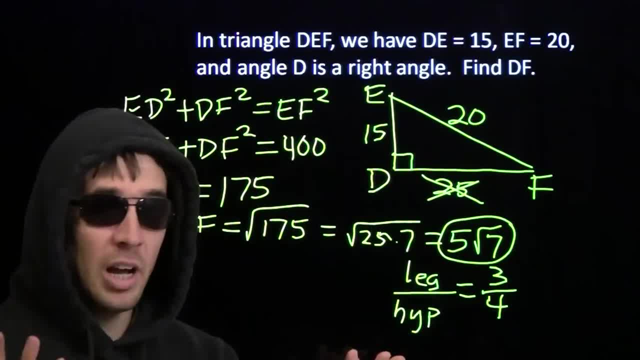 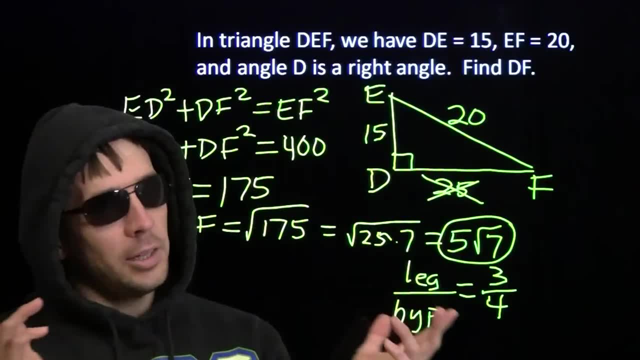 Still notice. if 15 and 20 have a common factor of 5, how could you still use that scaling strategy from the last video to solve this problem a little more quickly?